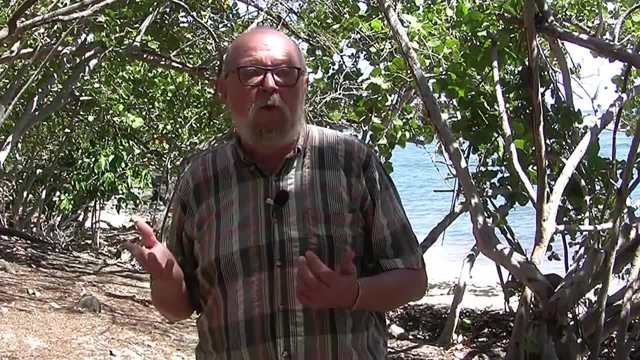 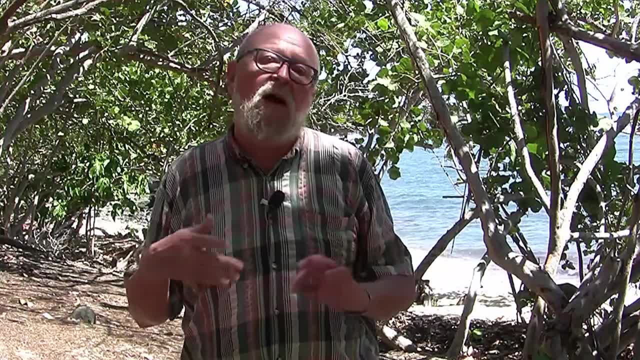 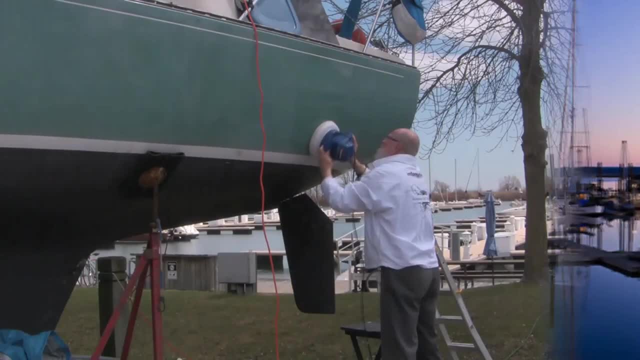 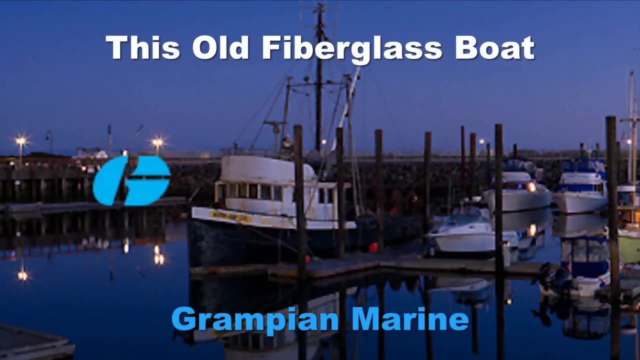 It also means that there will be about 1 tenth of an inch of rain or more in that particular period. It says nothing about how long the rain will last or how heavy it will be So, and it also says nothing about what happens next. 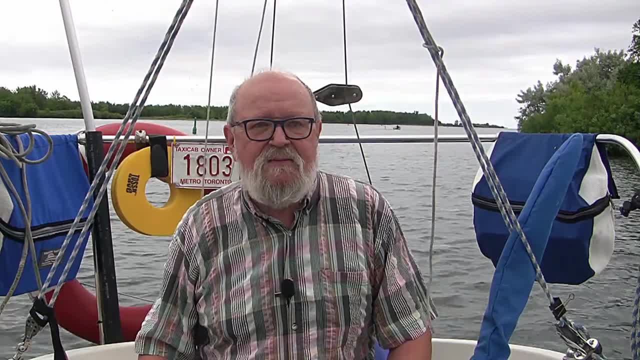 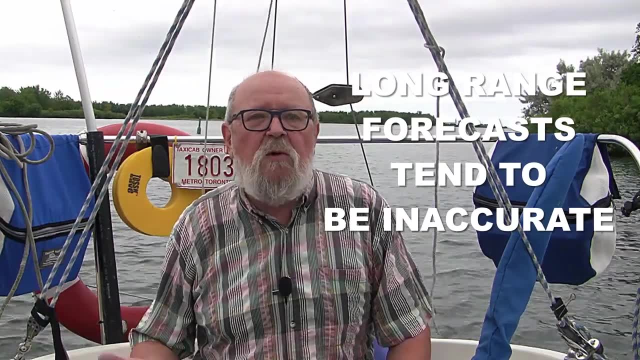 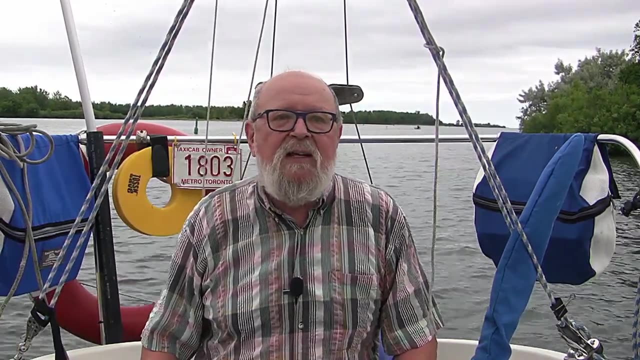 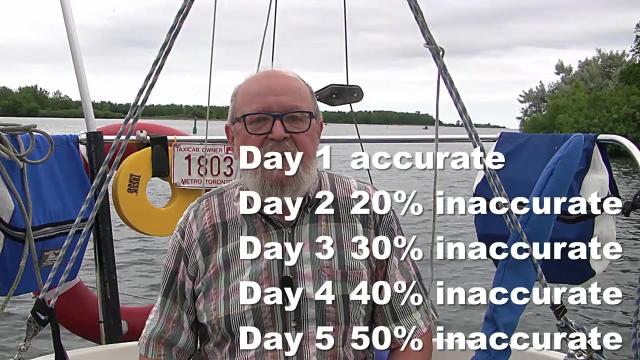 It says nothing about what happened in that day in the past. Also, the longer the forecast is, the lower the accuracy is Fairly accurate forecasts for the same day are quite reliable, But if you rely on a 5 day or less forecast every day, it's inaccurate by 10% or more a day. 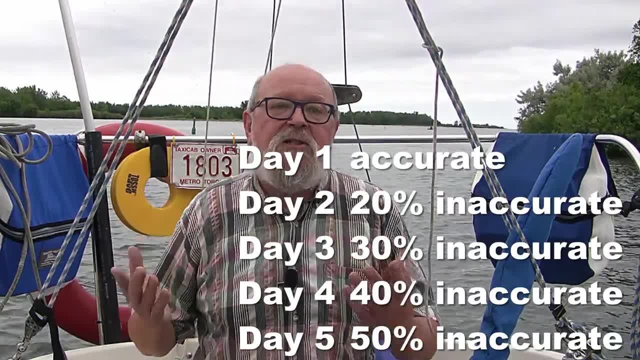 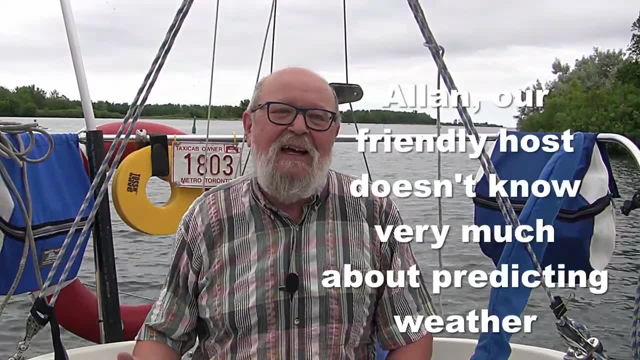 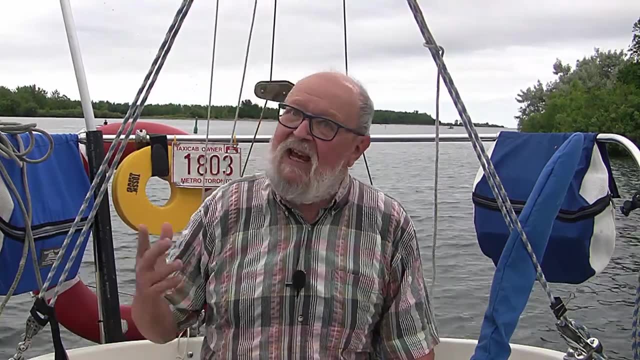 In addition to that, most TV weather people are not meteorologists, so they know about as much as I do Me. Now, there's no guarantee of accuracy, even when these forecasters use all the latest technologies, such as satellites and radar and Doppler. 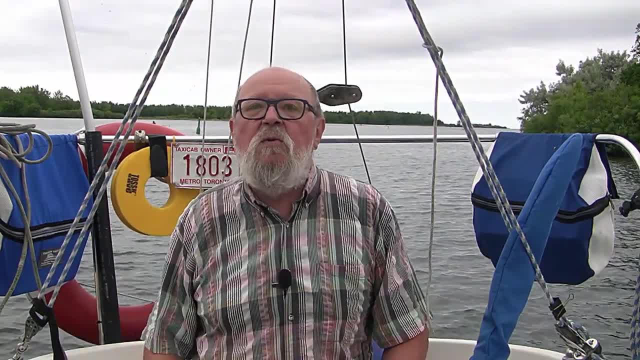 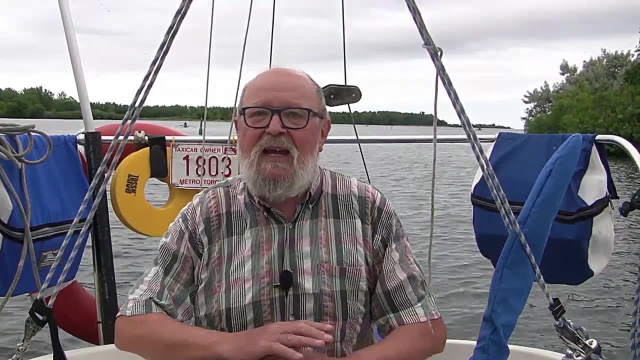 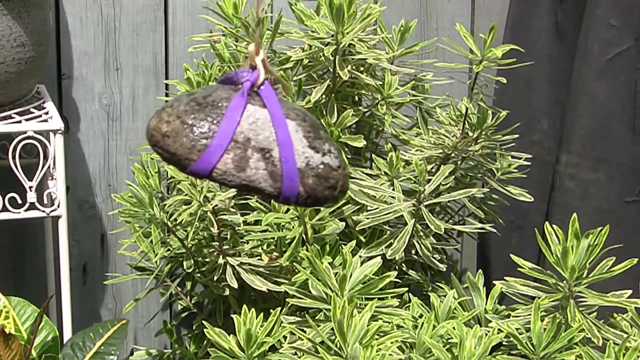 And there can be some amazing algorithms, but I have my own way of forecasting weather. My system has been used for centuries and is 100% accurate. I know what you're thinking. It's a weather rock. If the rock is wet, it's raining. If the rock is swinging, the wind is blowing. 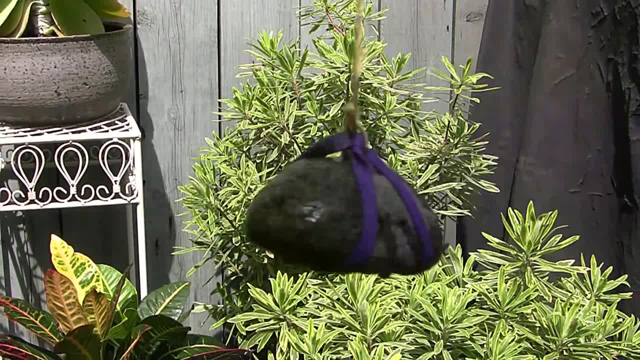 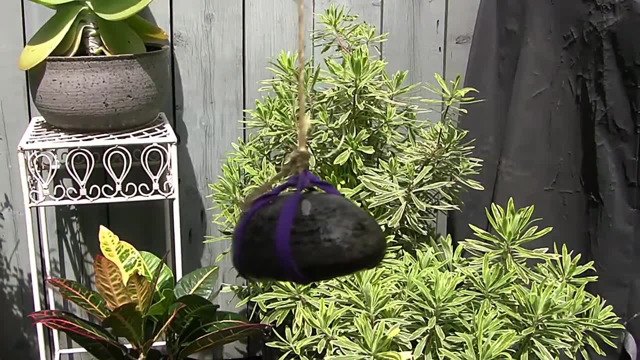 If the rock casts a shadow, the sun is shining. If the rock does not cast a shadow and is not wet, then the sky is just cloudy. If the rock is not visible, it must be foggy. By the way, I don't use a weather rock. 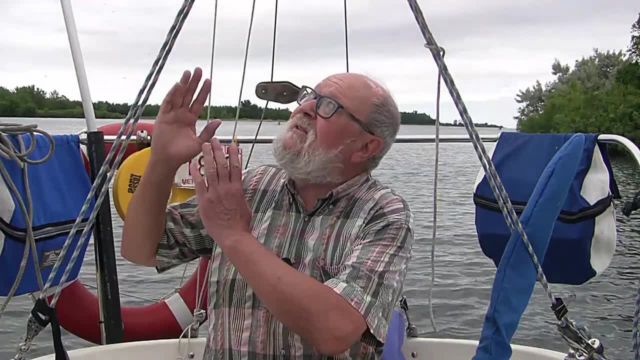 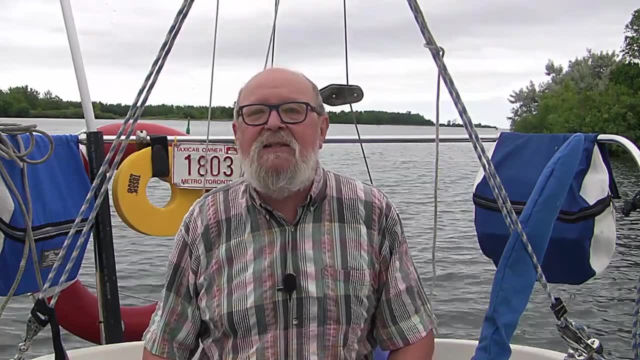 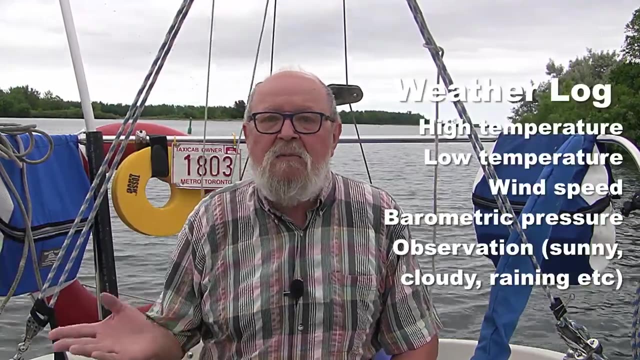 My predictions come from a higher source: The sky. It's a great way of supplementing your best weather forecast. Now you can do it too. I urge you to keep a weather log. Observe changes that you have observed during this weather log. 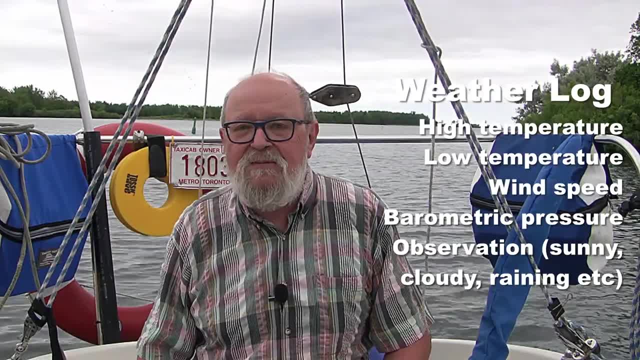 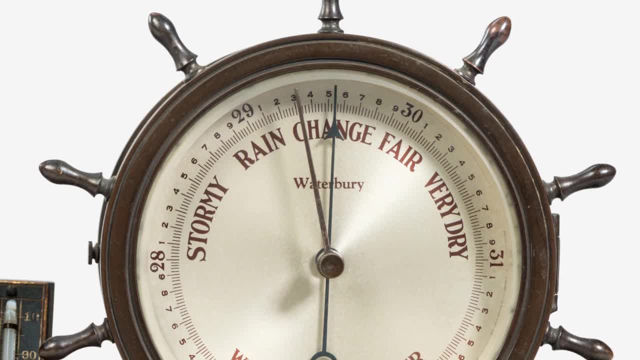 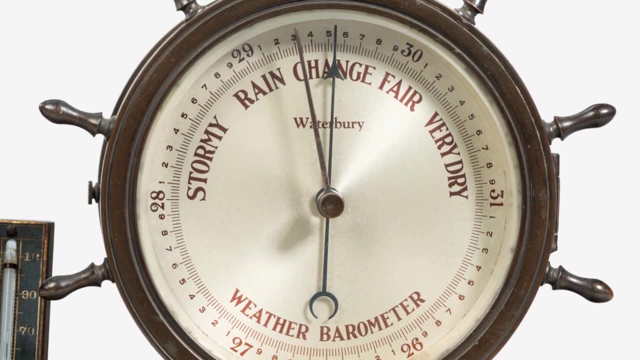 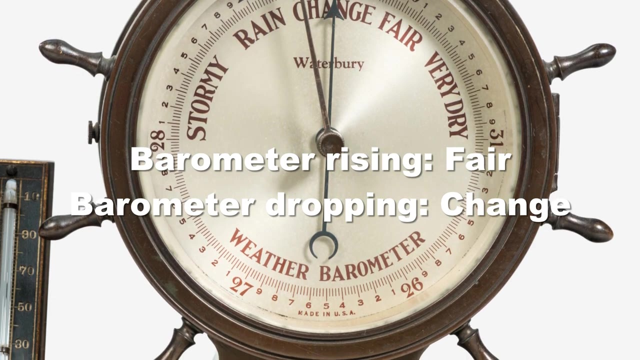 And it's even better if you have a barometer. The stormy, rain, change, fair, very dry markings was added to barometers in the early 20th century to try to sell them as weather predictors. In fact, it is the change or tendency that helps predict the weather, not the barometer. 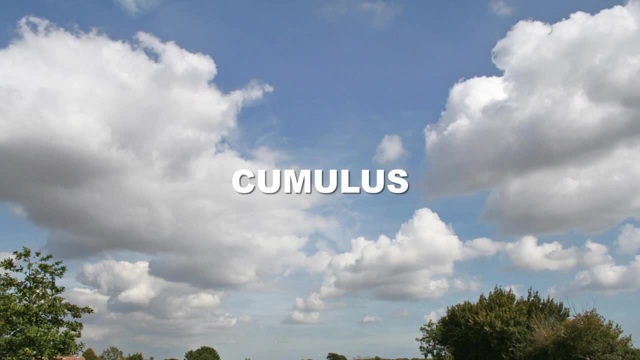 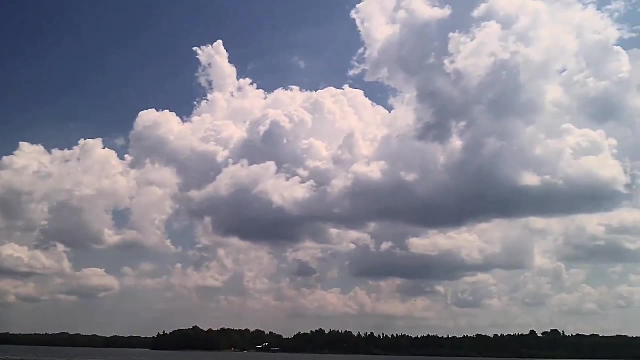 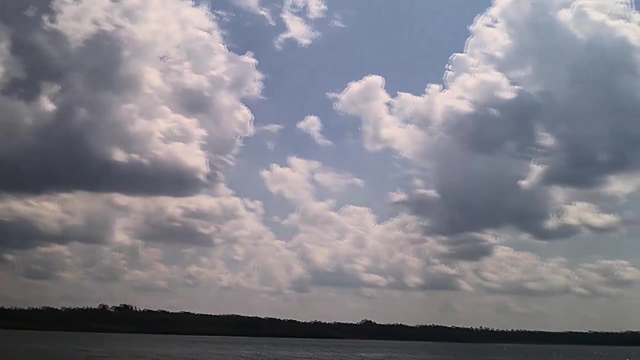 Here are a few cloud formations you will see in the next video. The northern hemisphere- Fair weather- cumulus. Normally, cumulus clouds produce little or no precipitation, but they can grow into the precipitation-bearing cumulimbus clouds. Stratus clouds usually predict poor weather is coming. 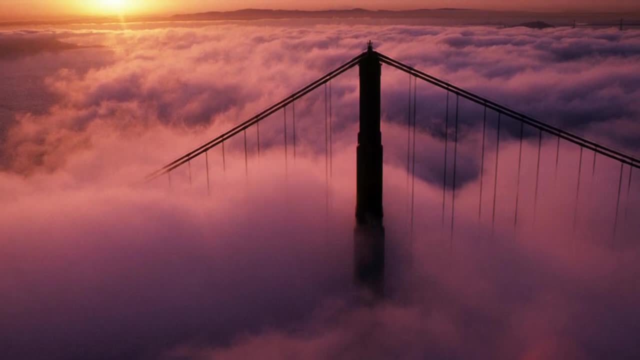 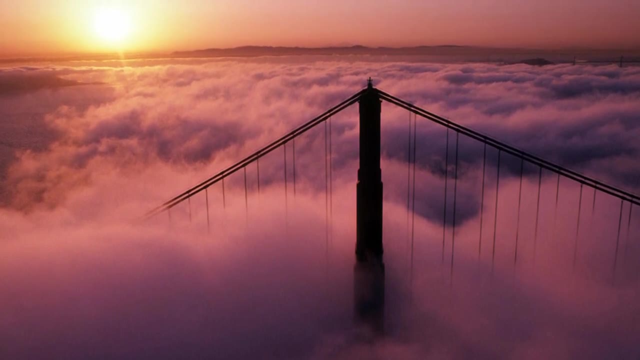 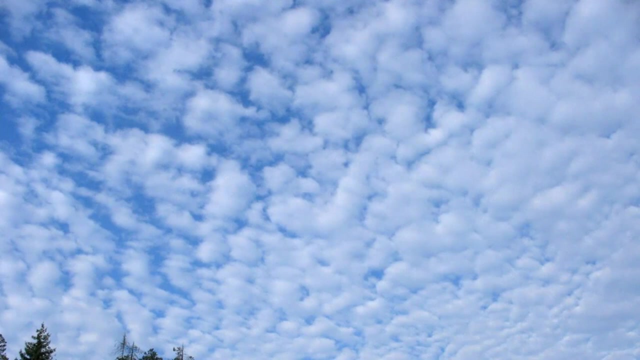 These clouds are essentially above-ground fog that forms either through the lifting of morning fog or through cold air moving at low altitudes over a region. They also can forecast light rain Stratocumulus. These clouds are low, lumpy and grey. 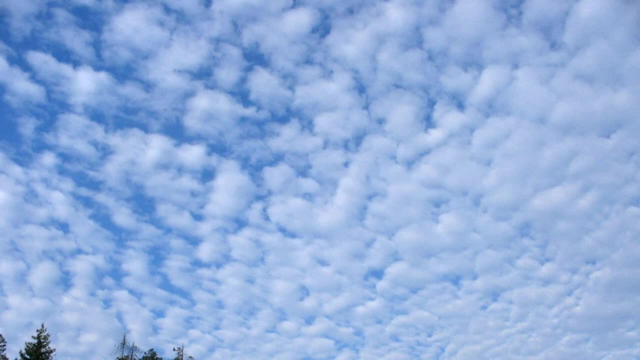 These clouds can look like cells under a microscope. They may look like fist scales, And sometimes they line up in rows and other times they spread out. Only light precipitation, generally in the form of drizzle, occurs with stratocumulus clouds. 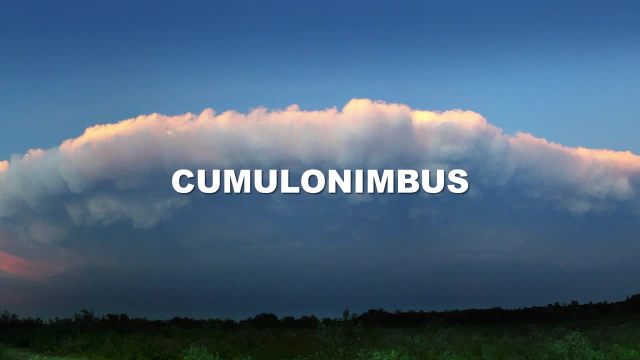 Cumulonimbus. They are generally known as thunderstorm clouds. A cumulonimbus cloud can grow up to 10 km high. At this height, high winds will often flatten the top of the cloud out to make it look like it is anvil-shaped. 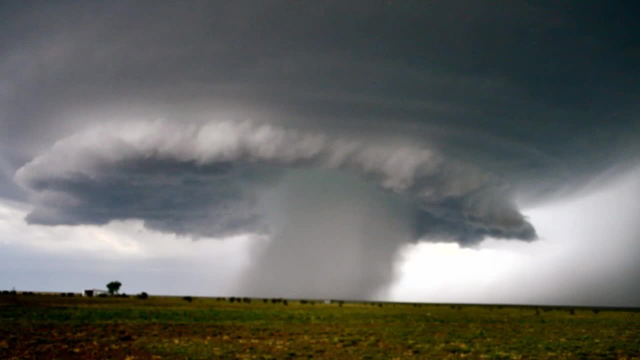 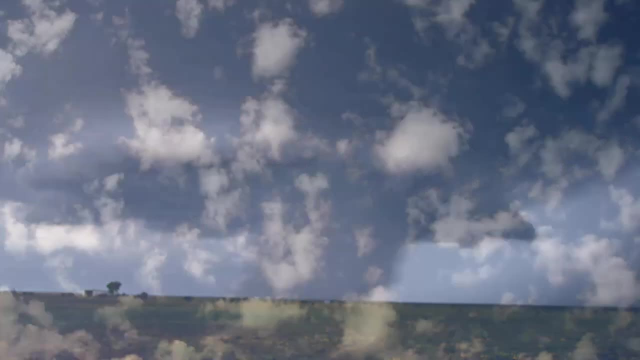 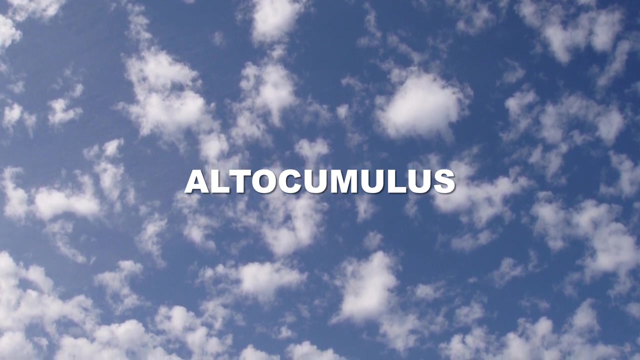 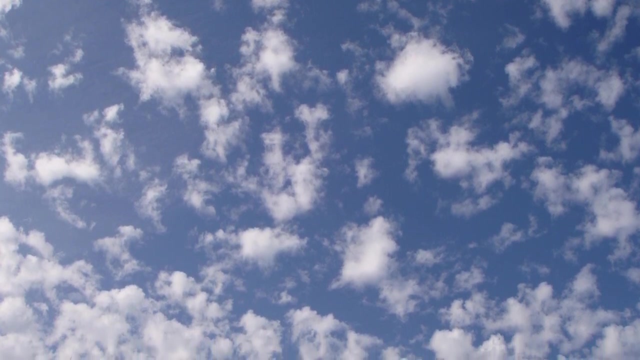 Cumulonimbus clouds are associated with heavy rain, hail, lightning and tornadoes. Watch out for these. Altocumulus clouds are greyish-white, with one part of the cloud darker than the other. Altocumulus clouds usually form in groups and are about 1 km thick. 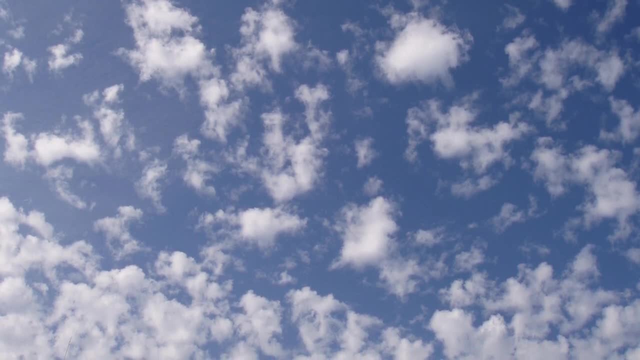 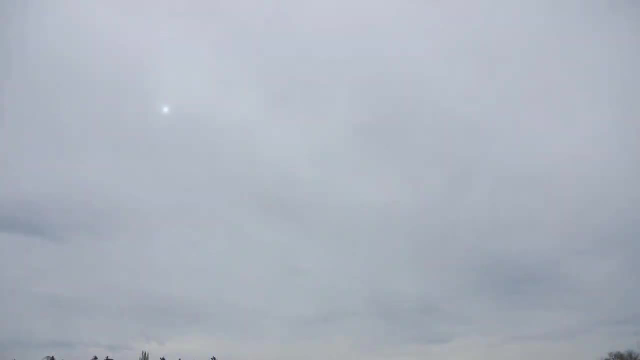 If you see these altocumulus clouds on a warm, humid morning, then expect thunderstorms by late afternoon. Altostratus clouds usually cover the whole sky and have grey or blue-grey appearance. The sun or moon may shine through as an altostratus cloud, but will appear rather watery or fuzzy. 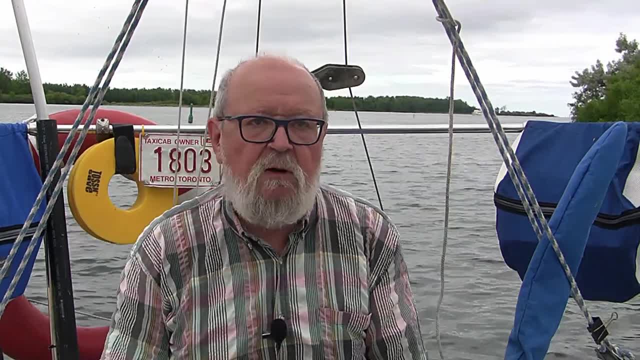 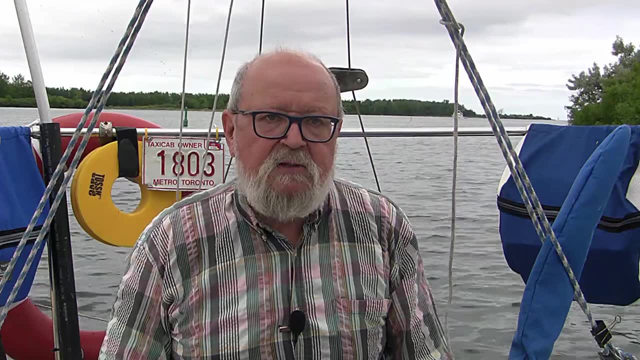 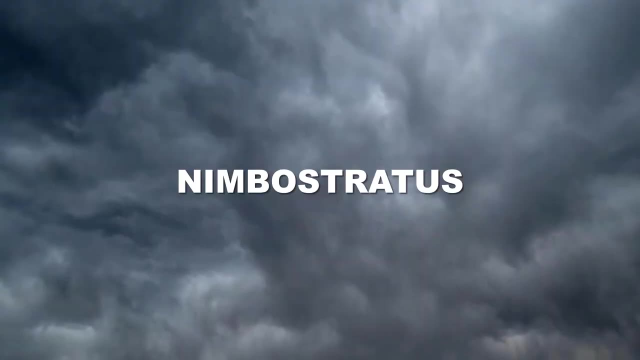 An altostratus cloud usually forms ahead of a storm that has continuous rain. Occasionally, the rain will fall from an altostratus cloud, But if the rain hits the ground, then the cloud becomes classified as a nimbostratus cloud. Nimbostratus are dark grey with a ragged base. 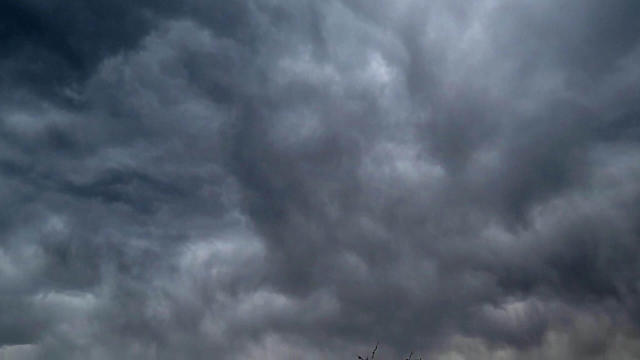 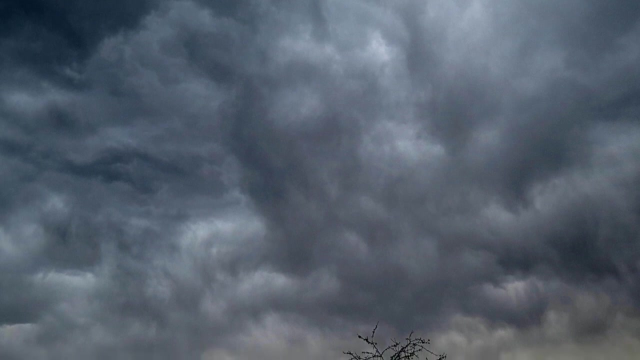 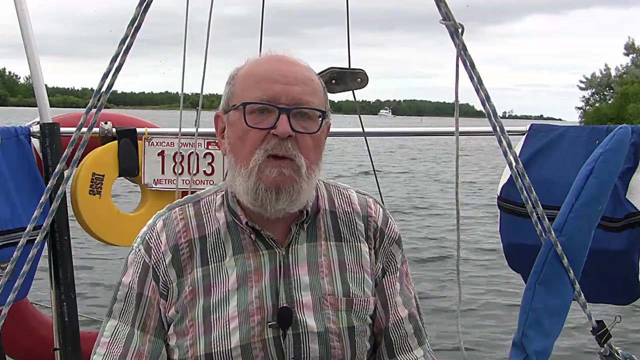 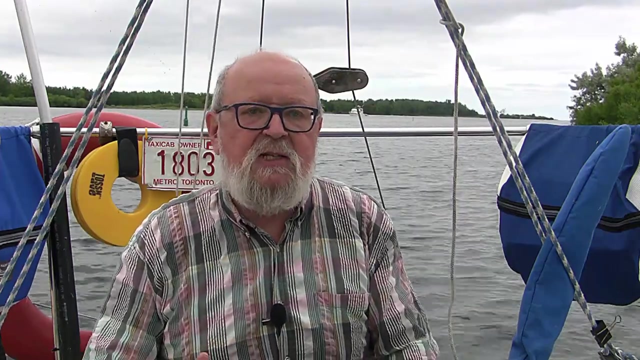 Nimbostratus. clouds are associated with continuous rain. Sometimes they cover the whole sky and you can't even see the edges of the cloud. You can tell where the weather will come from by observing wind direction and the barometric pressure. Wind direction changes often and it's accompanied by changes in the weather. 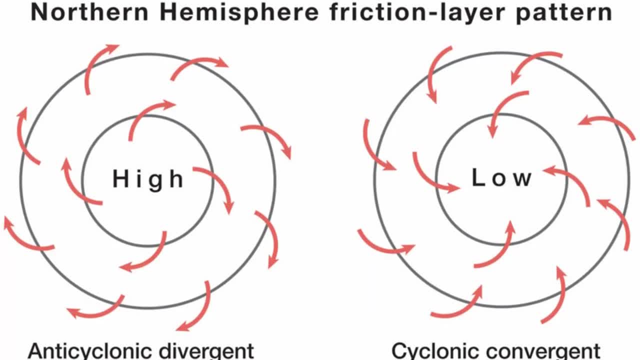 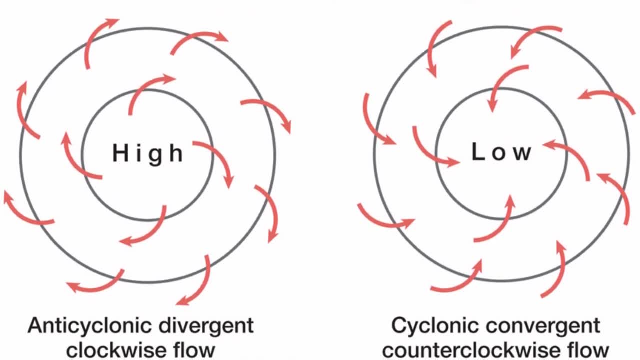 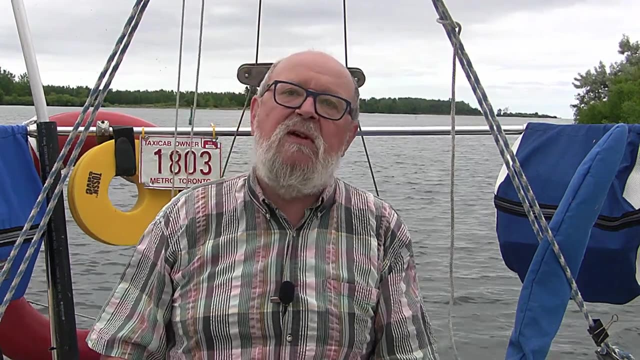 The air flows cyclonically around a pressure system. If the wind changes direction in a cyclonic fashion, it often means low pressure or a front is influencing the area. A wind shifting from the south, for instance, means warmer air is approaching. 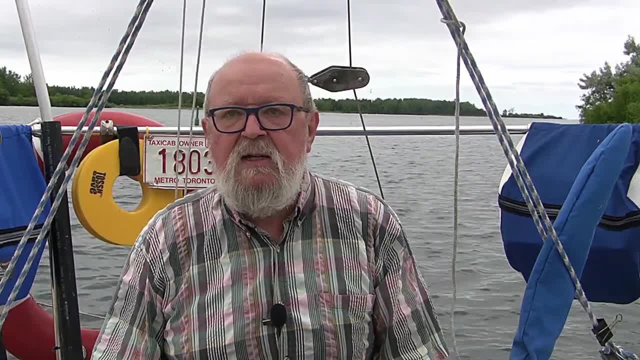 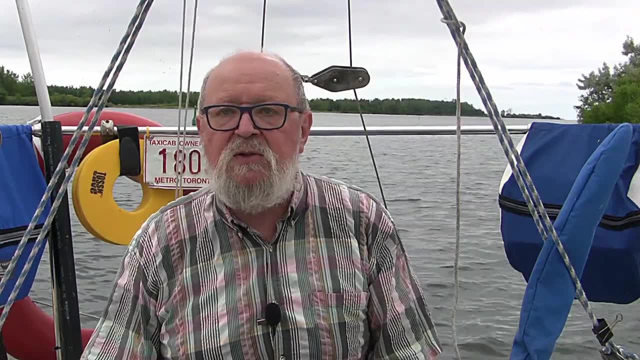 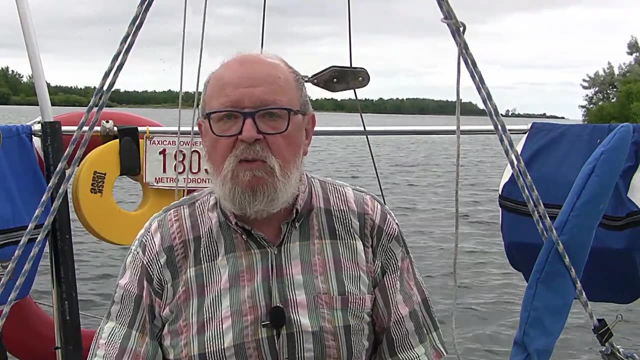 And wind from the north often means cooler air is approaching. When the wind changes abruptly, it could be a frontal passage or wind direction change caused by a thunderstorm. As a rule, in my area, winds from the east quadrant and falling barometric pressure indicate foul weather. 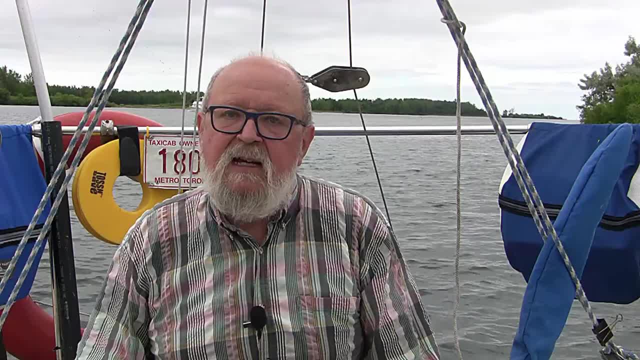 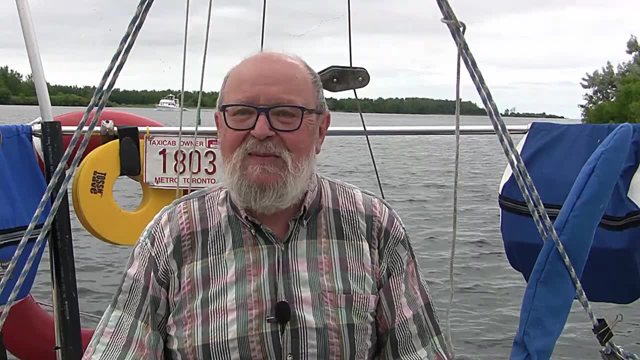 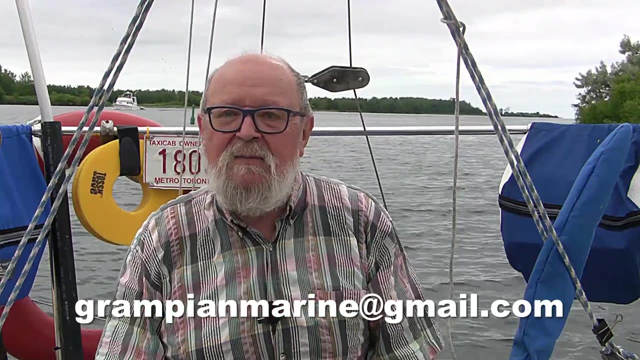 And winds shifting to the western quadrant indicate clearing and fair weather, But there are exceptions, So that's it. I'd love to hear your comments and suggestions. Please type them below Or you can email me. Give me a thumbs up And subscribe.